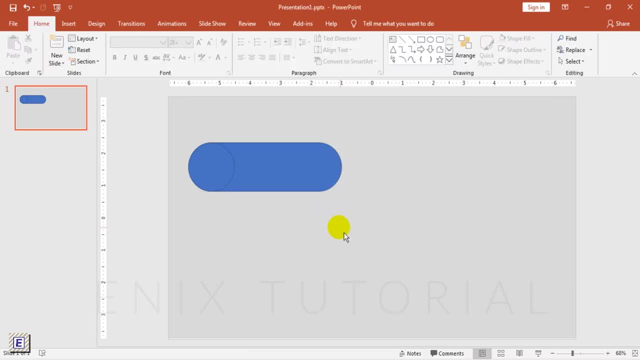 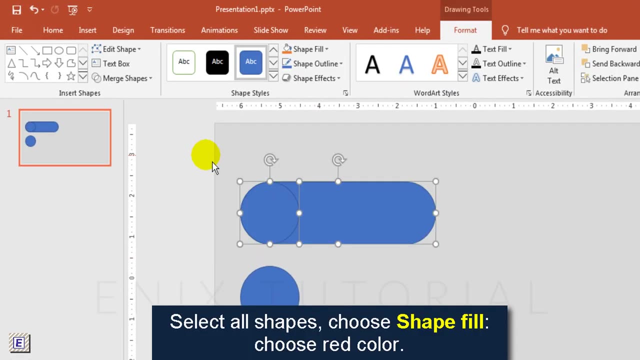 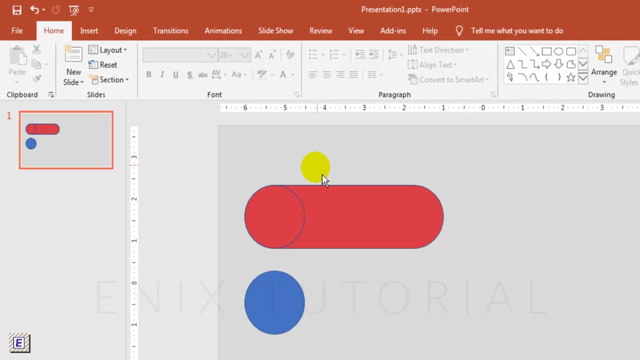 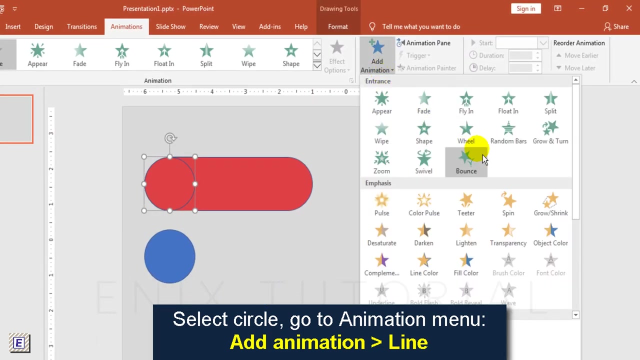 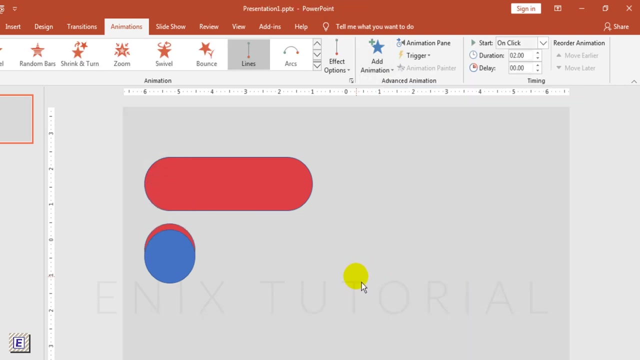 Right click choose send to back Select circle. press control D to duplicate circle. Select all shapes. choose shape Fill. Choose red color. Select circle. Go to animation menu. Add animation. Choose line Effect options. choose right. 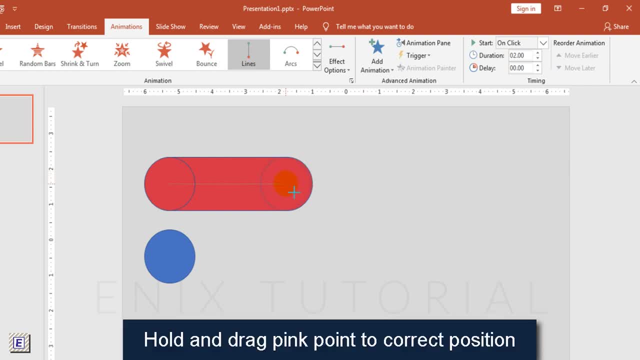 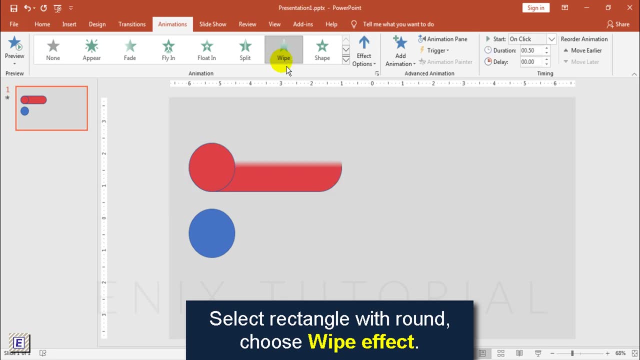 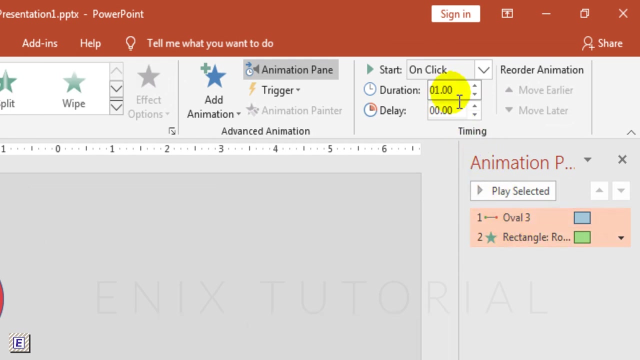 Hold and drag pink point to correct position. select rectangle with round. Choose wipe effect Effect option. choose from left: Click animation pain. Hold shift button. select effects 1 and 2.. Duration: 1 second. Select effect 2, choose. start with previous. 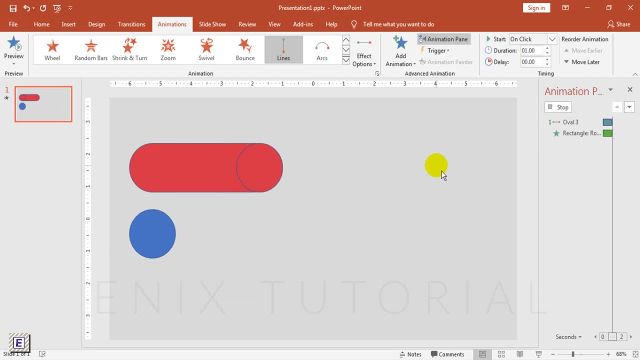 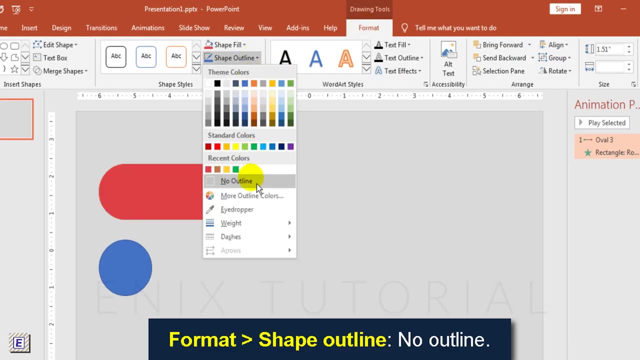 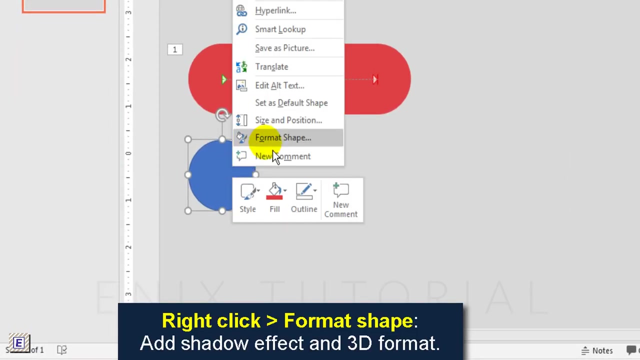 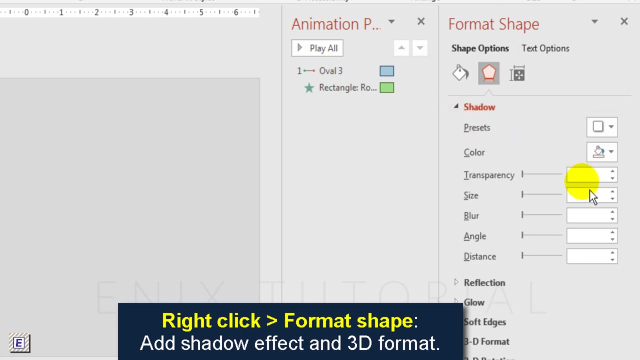 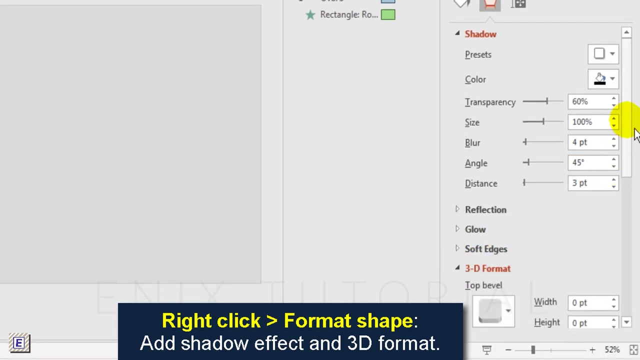 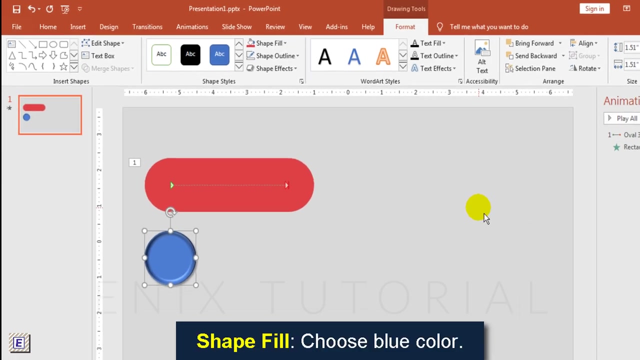 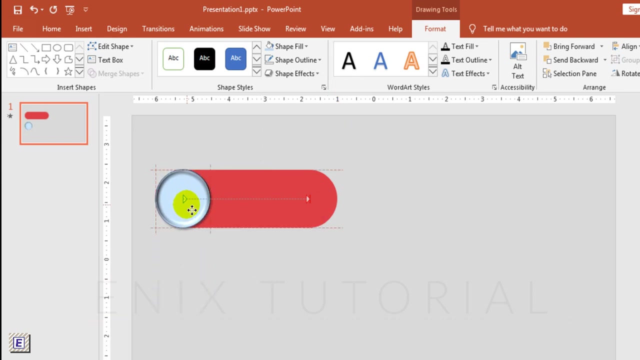 Heateschain feature of hatch 2 on screen. Select Pink Color Shapes. Format Shape: Outline: choose No Outline. Right-click: choose Format Shape. Now I will add shadow effect in 3D format Shape Fill: choose Blue Color. Move this circle to same position with Pink Shape. 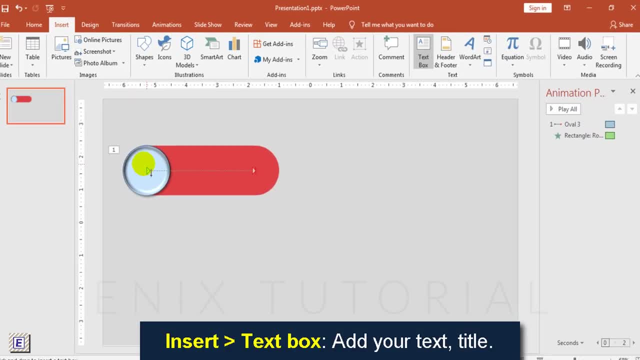 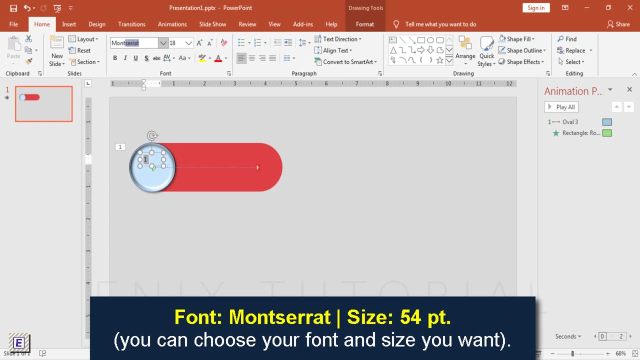 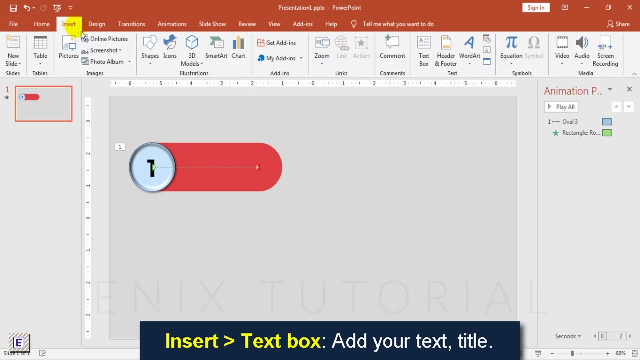 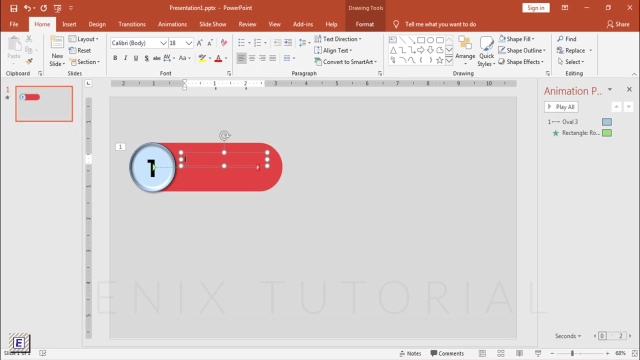 Insert Text Box to add your title and text. I choose Font: Montserrat. Size: 54 pt. You can choose any font and size you want. Insert Text Box. then add text title. Select Text. Go to Animation Menu. choose Wipe Effect. 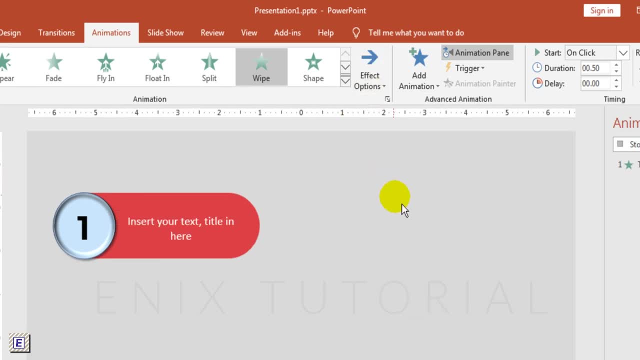 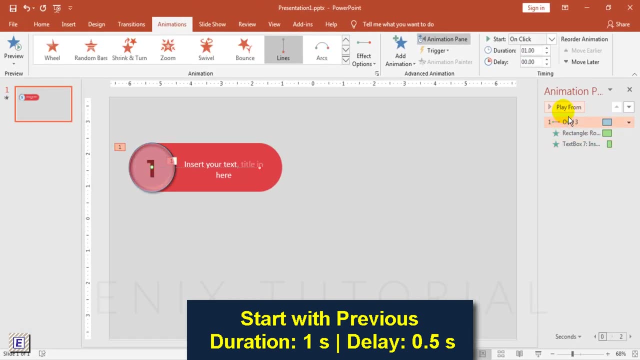 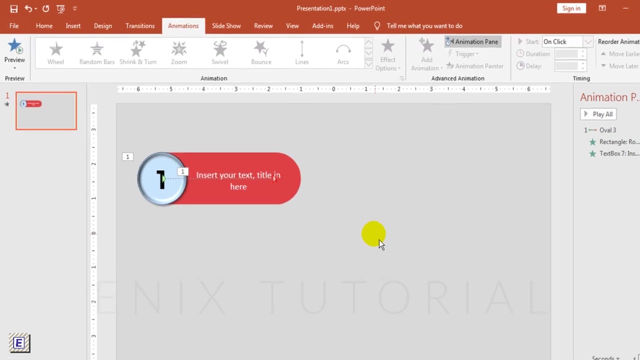 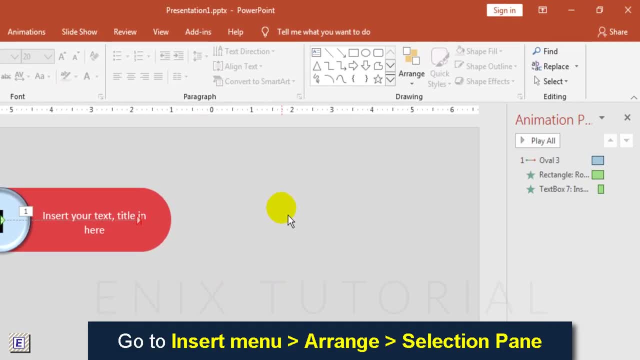 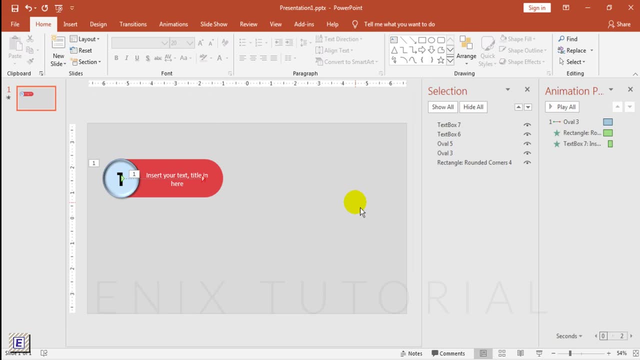 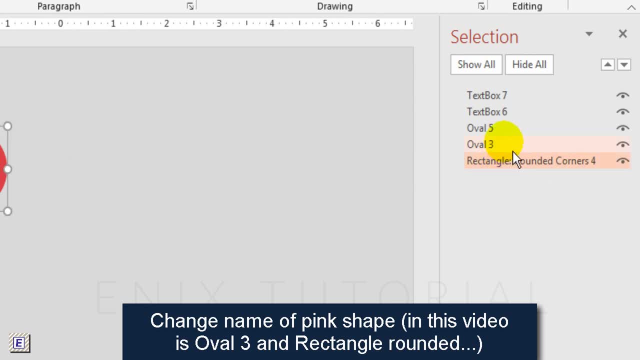 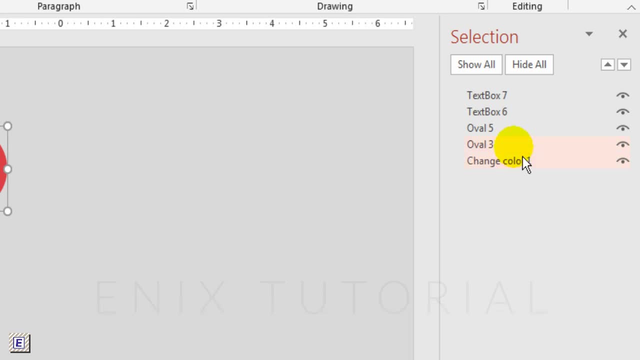 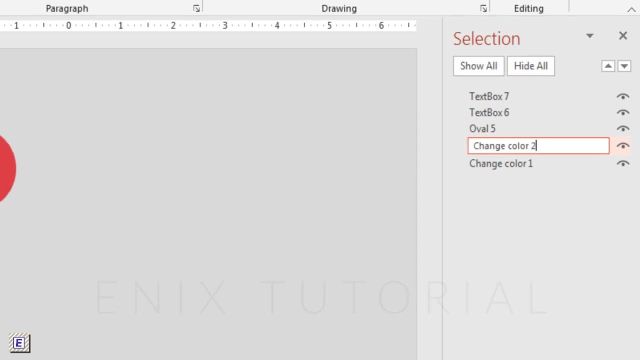 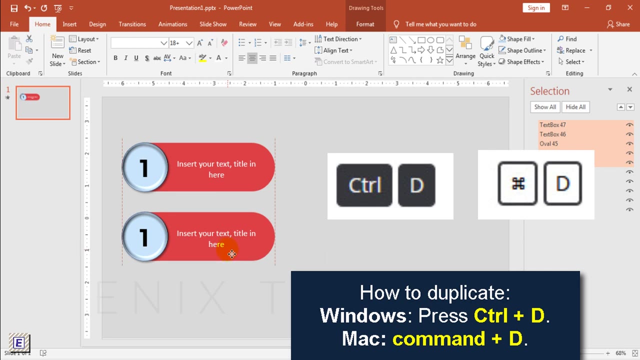 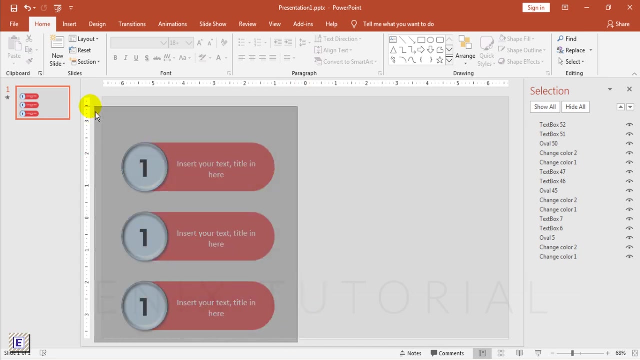 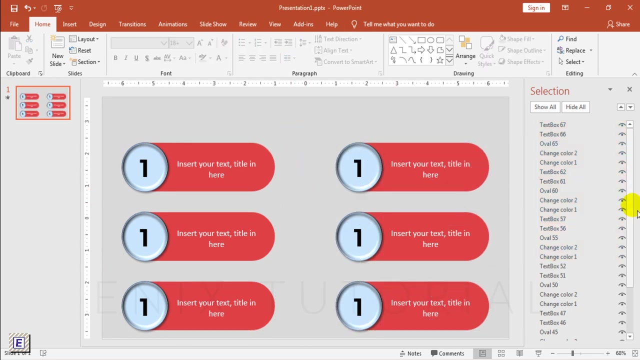 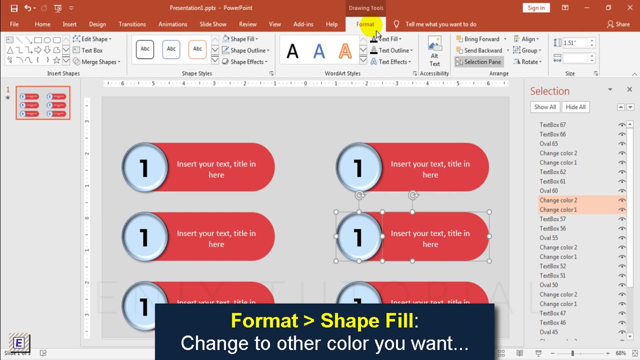 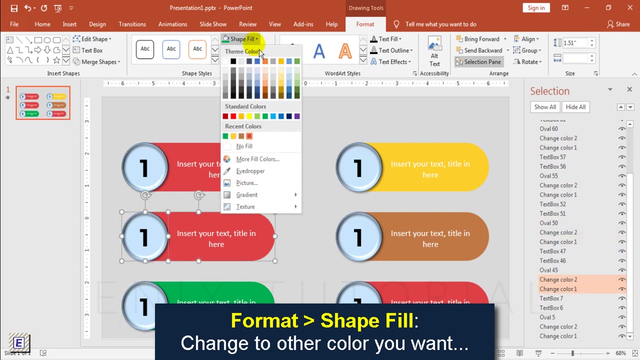 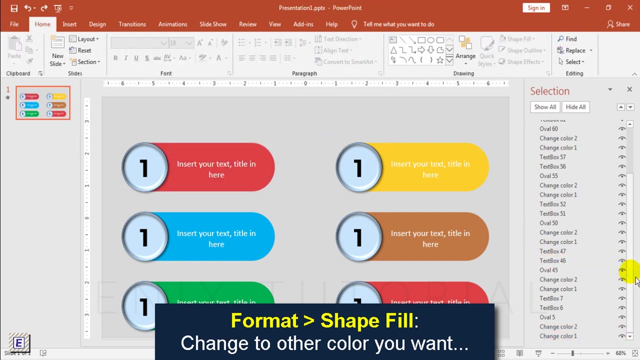 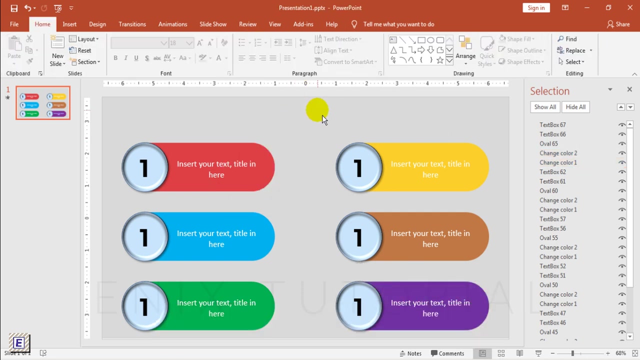 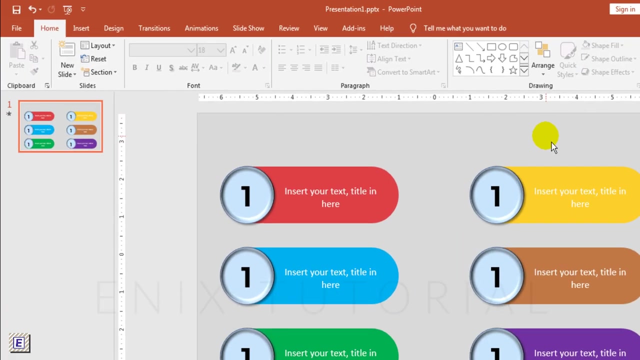 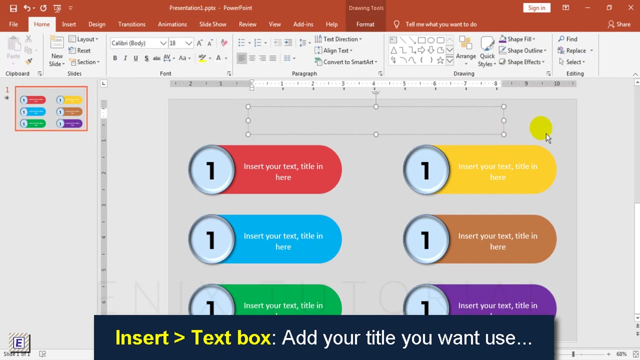 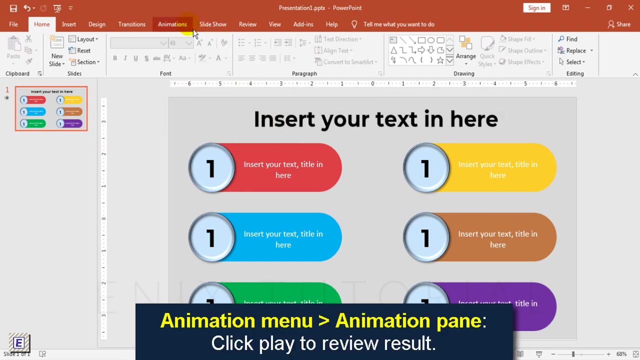 Select the text. Select all shapes, then duplicate shapes. Hold shift button. select pink shapes. Go to format menu. choose shape fill, then choose color. you want. use Insert text box to add text title. you want Change font name size. Animation menu: click on the animation pane.